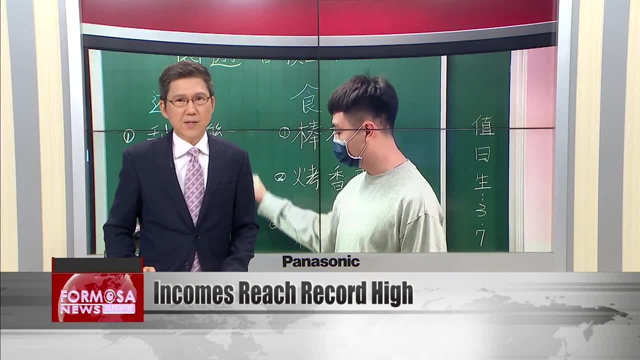 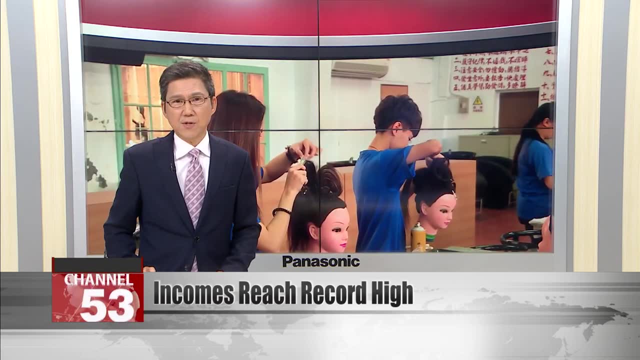 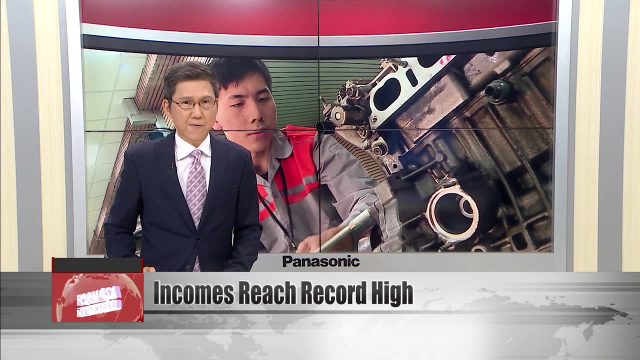 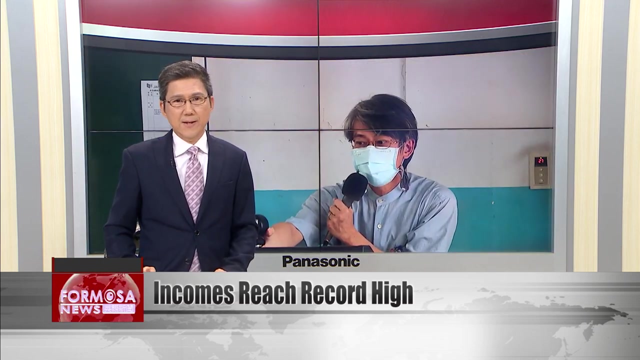 salary increases. The highest-earning industries continue to be traditional jobs for life, such as education, the military and civil service, finance and insurance, But as higher education becomes more and more the norm, the survey also revealed that vocational college grads earn on average, more than university alumni. Some analysts are saying that the value 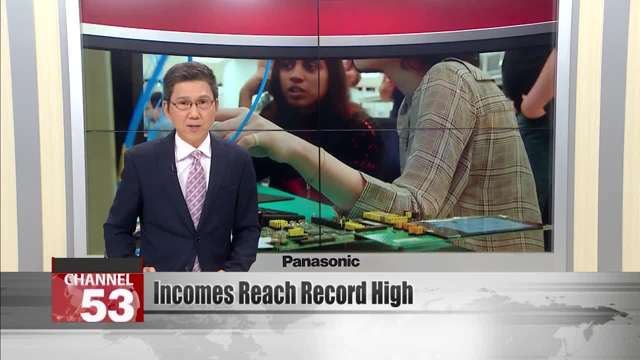 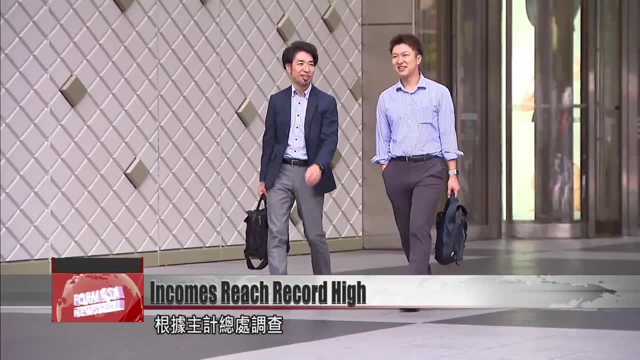 of a bachelor's degree is no longer what it once was. A survey by the Directorate General of Budget, Accounting and Businesses said that the value of a bachelor's degree is no longer what it once was. Statistics found that the average Taiwanese annual income for 2022 was 700,000 NT, a new record. high. There were also new records set for incomes in all different age brackets: For under-30s, 535,000 NT a year or 44,000 NT a month. The highest-earning age group is 45 to 54-year-olds. 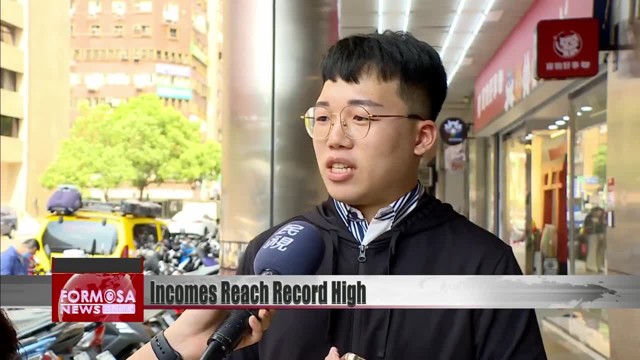 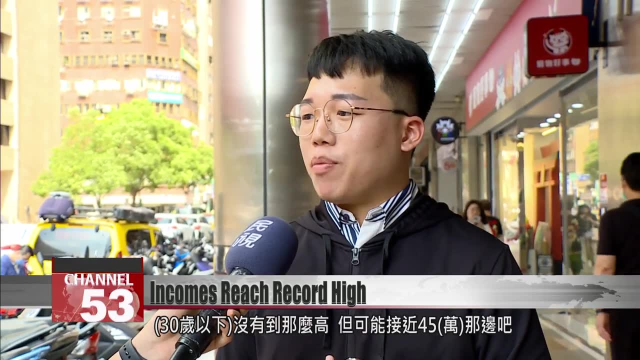 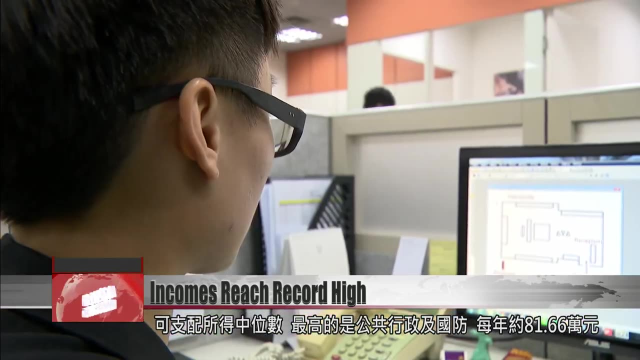 at more than 900,000 NT a year. People aged 45 to 54, are probably all at managerial levels or above. People under 30 haven't reached that high, but they're probably reaching 450,000 NT. The median disposable income varies by industry. 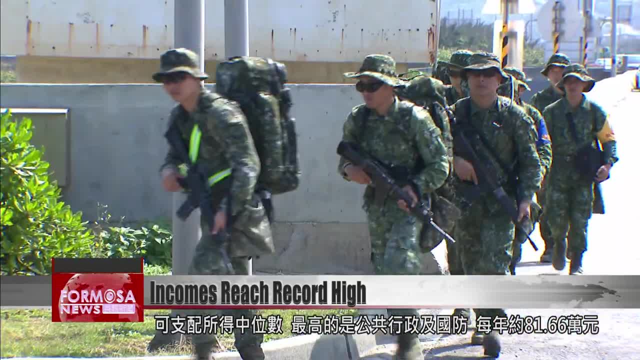 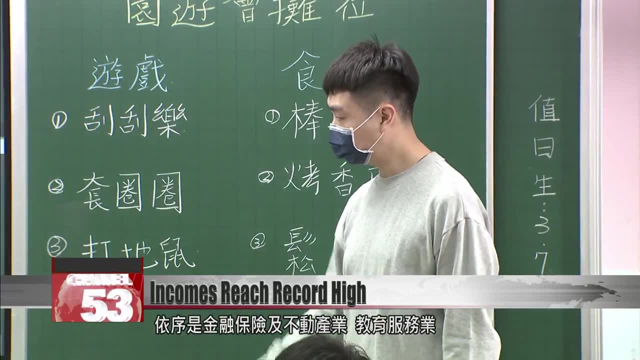 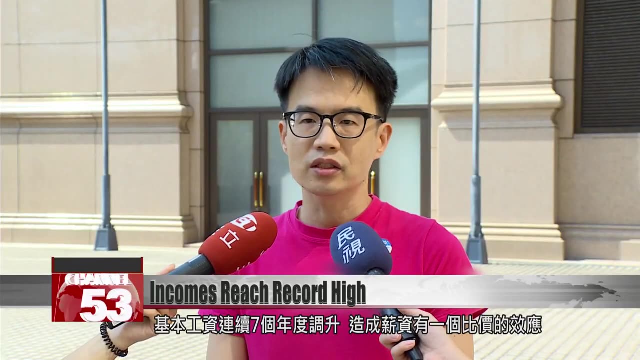 The highest disposable incomes are commanded by those in public administration and national defense, with 816,000 NT a year on average. After that, the top industries are finance and insurance, real estate and educational services. The basic income has gone up for seven years in a row. The average income for a bachelor's degree is about $1,000 a year. 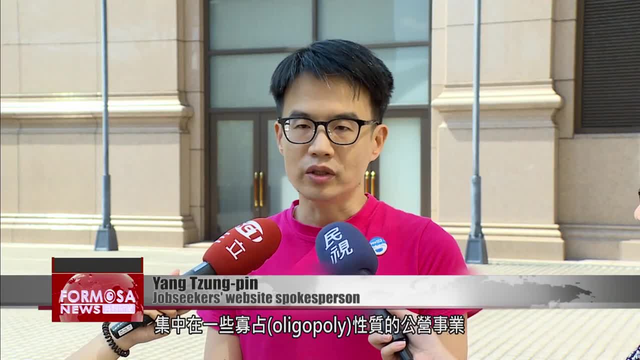 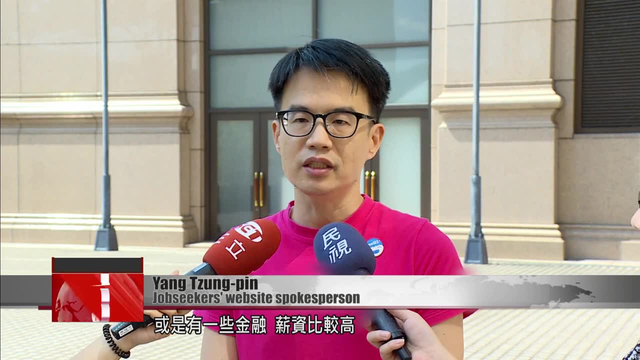 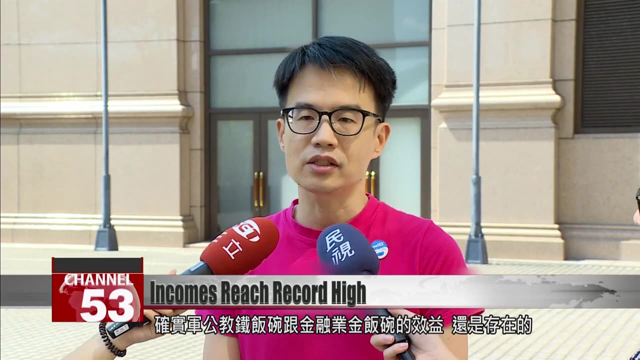 Which has caused salaries to become more competitive. There are higher salaries in finance and in certain publicly-owned enterprises which have some of the characteristics of oligopolies. So indeed, there's still the job security of the iron rice bowl- military, civil service and education jobs- and the golden rice bowl of finance. 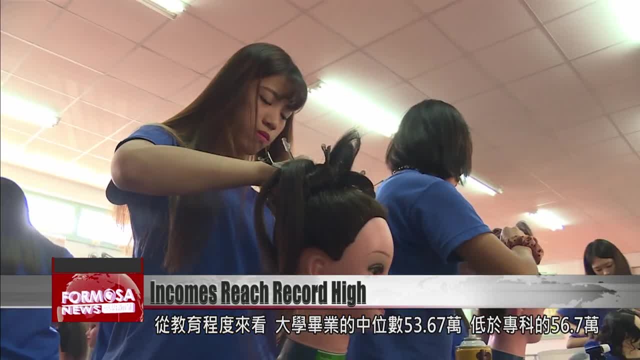 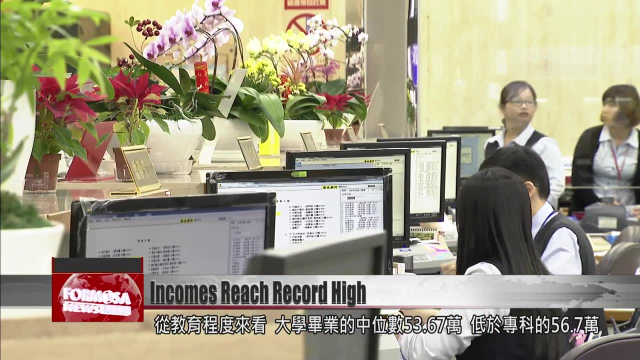 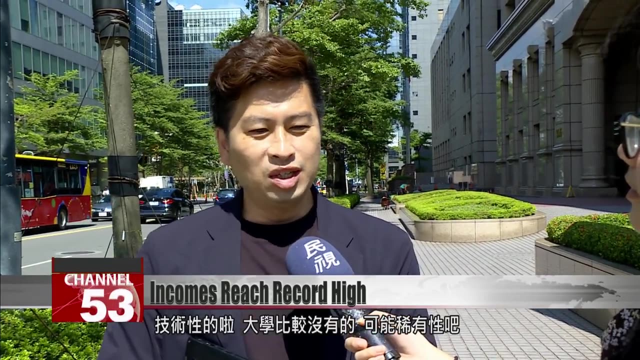 So which qualifications pay off? Well, university graduates have a median income of 536,000 NT, less than the graduates of vocational colleges at 536,000 NT. They have technical skills that university grads don't. Perhaps it's because the skills 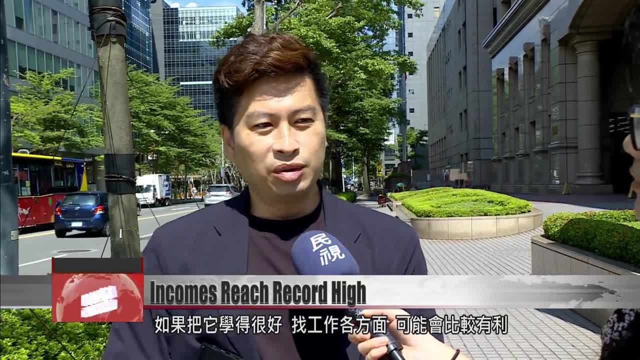 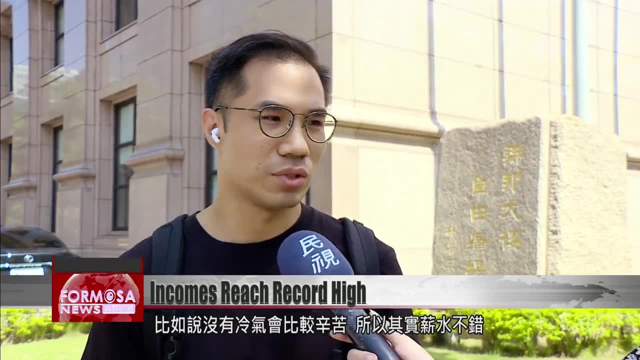 are rare. If you learn it well, it can be very beneficial in the job search all around. For example, they have to work without air con, so it's hard work and the salary is good, but many people might think it's too tough and wouldn't be willing to do it.